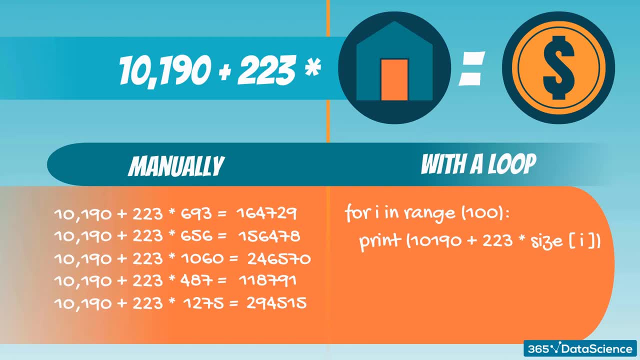 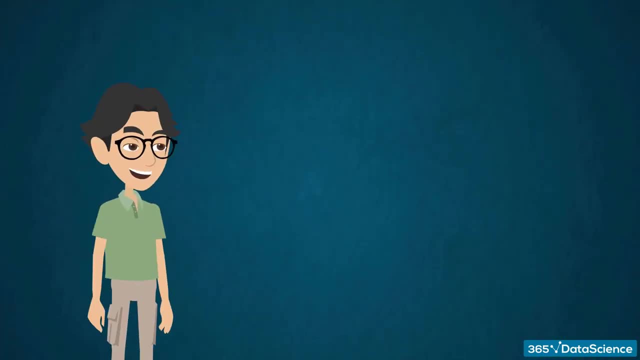 sizes, multiplying each of them by 223 and adding 10,190.. However, we are smarter than that, aren't we? We know some linear algebra already. Let's explore these two objects: A 5 by 2 matrix and a vector of length 2.. The matrix contains a column of 1s and another. 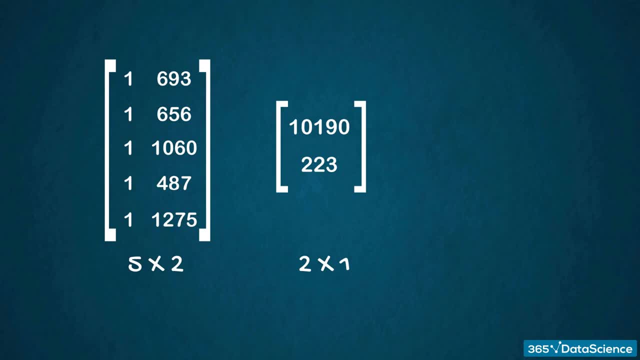 with the sizes of the houses. The vector contains 10,190 and 223, the numbers from the equation. If we go about multiplying them, we will get a vector of length 5.. The first element will be equal to 1 times 10,190 plus 695.. The first element will be equal to 1 times 10,190 plus 695.. 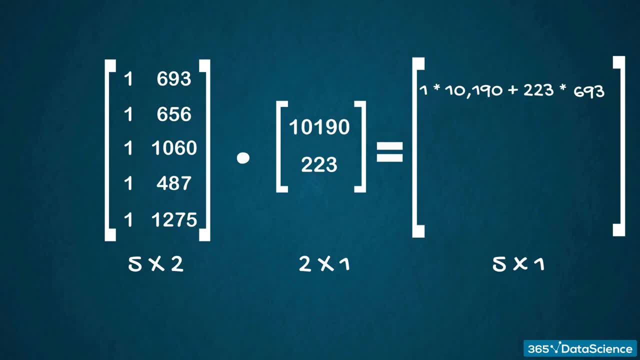 The second element will be equal to 1 times 10,190 plus 696 times 223.. The second two: 1 times 10,190 plus 656 times 223.. And so on. By inspecting these expressions, we quickly realize that the resulting vector contains: 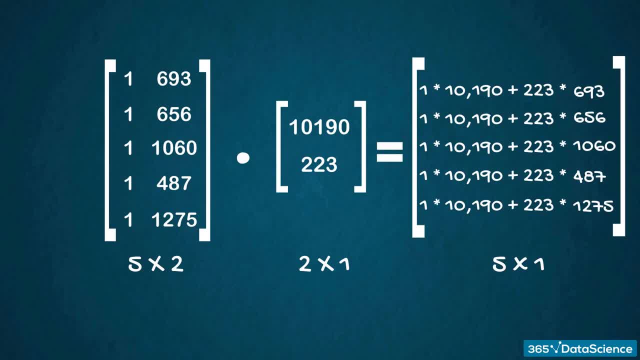 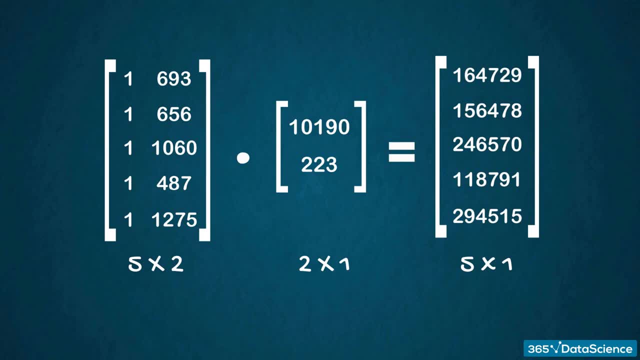 all the manual calculations we made earlier to find the prices In machine learning, and linear regressions in particular. this is exactly how algorithms work. We've got an inputs matrix, a weights or a coefficients matrix and an output matrix. Without diving too deep into the mechanics of it here, let's note something. 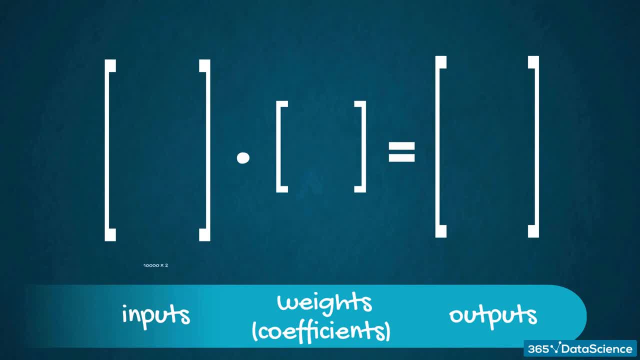 If we have 10,000 inputs, the initial matrix would be 10,000 by 2, right, The weights matrix would still be 2 by 1.. When we multiply them, the resulting output matrix would be 10,000 by 1.. This shows us that, no matter the number of inputs, we will get just 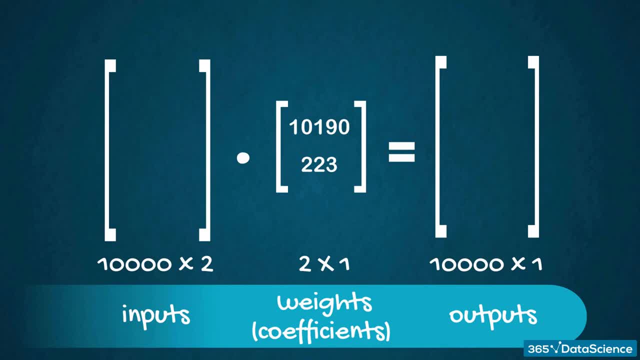 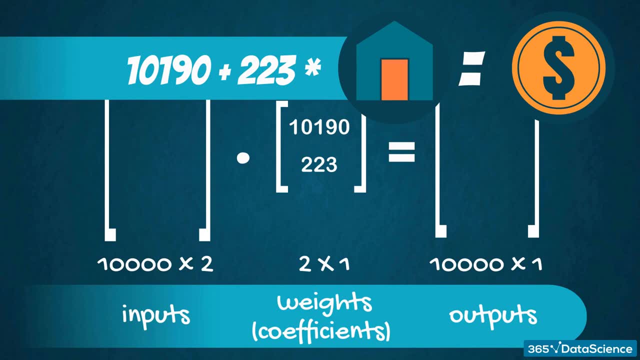 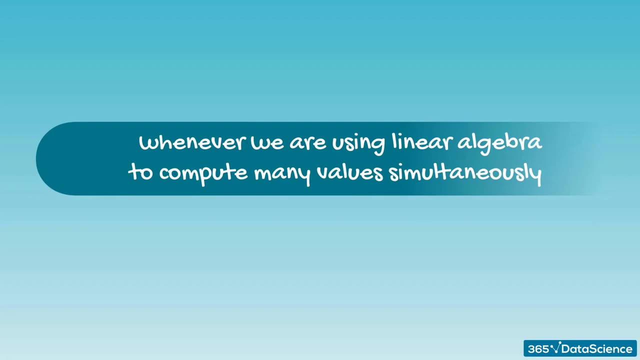 as many outputs. Moreover, the equation doesn't change, as it only contains the two coefficients 10,190 and 223.. All right, So whenever we are using linear algebra to compute many values simultaneously, we call this array programming or vectorizing code. 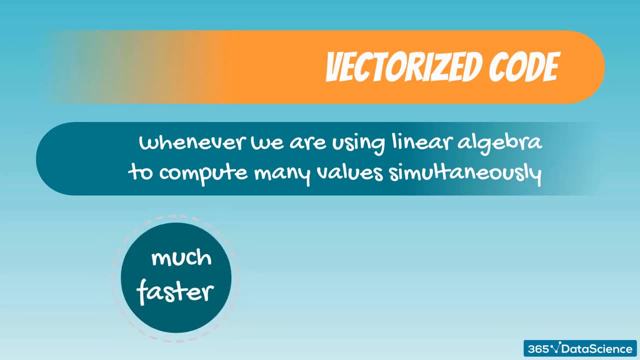 It is important to stress that array programming is much, much faster. There are libraries, such as NumPy, that are optimized for performing this kind of operations, which greatly increases the computational efficiency of our code. Okay, What about image recognition In the last few years? deep learning, 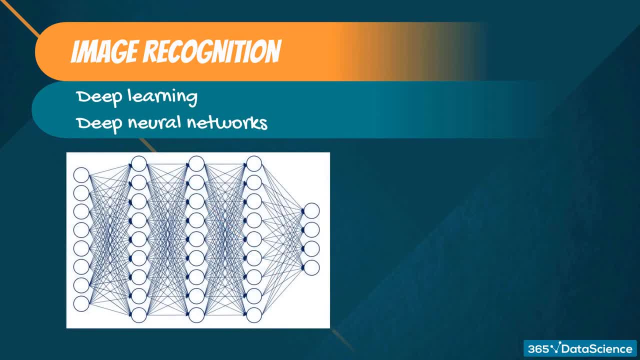 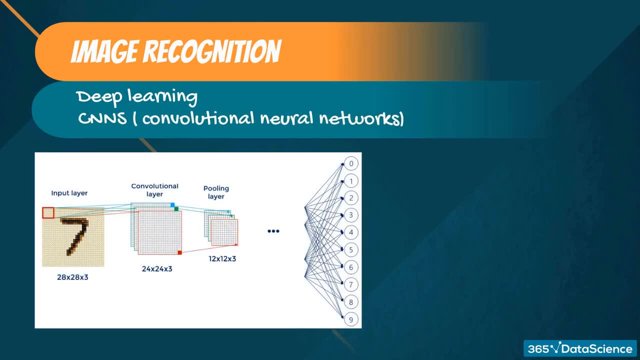 and deep neural networks, in particular conquered image recognition. On the forefront are convolutional neural networks, or CNNs. in short, What is the basic idea? You can take a photo, feed it to the app and send it to your computer. You can also take a photo, feed it to the app and send it to your computer. 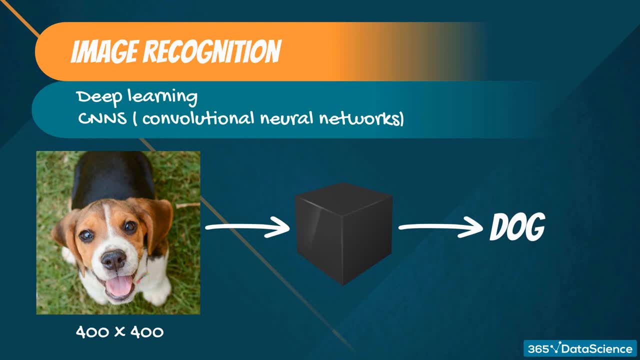 You can also take a photo, feed it to the app and send it to your computer. You can also take a photo, feed it to the app and send it to your computer And classify it. Famous examples are the MNIST dataset, where the task is to classify. 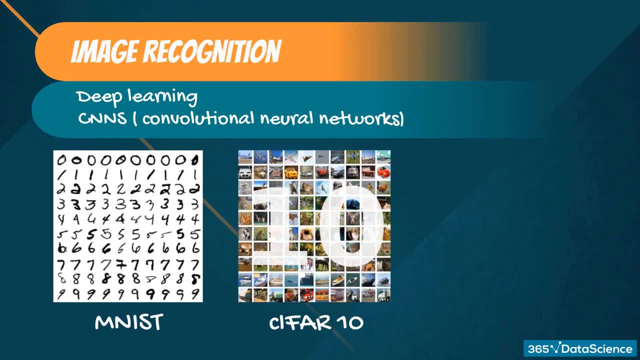 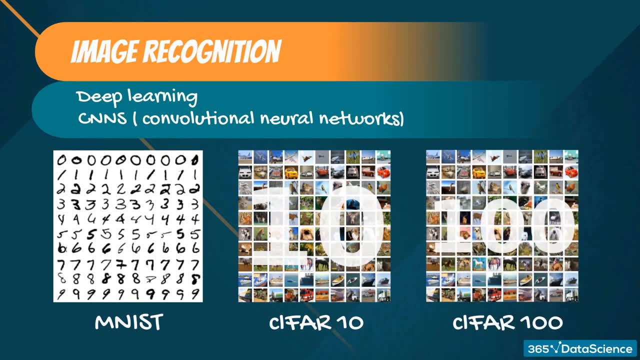 handwritten digits: CIFAR-10,, where the task is to classify animals and vehicles, and CIFAR-100,, where you have 100 different classes of images. The problem is that we cannot just take a photo and give it to the computer. 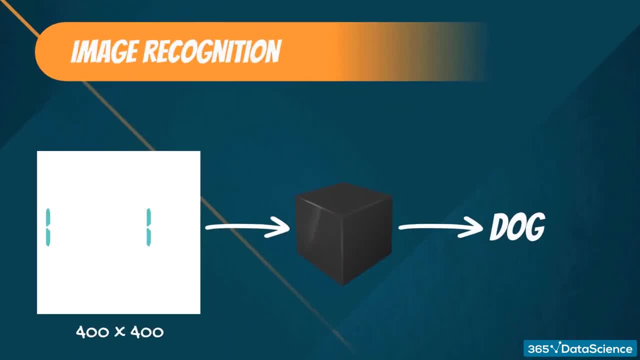 We must design a way to turn that photo into numbers in order to communicate the image to the computer. Here's where linear algebra comes in. Each photo has some dimensions, right? Say, this photo is 400 by 400 pixels. Each pixel in a photo is basically a colored square. 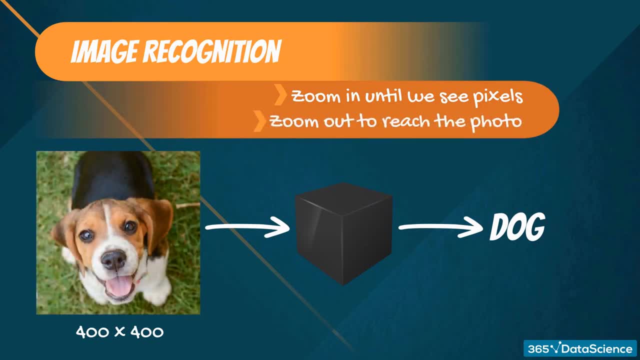 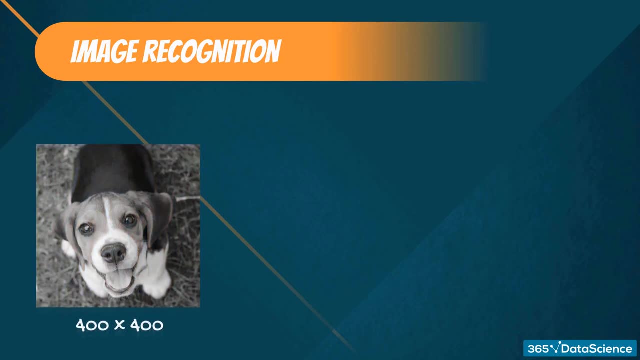 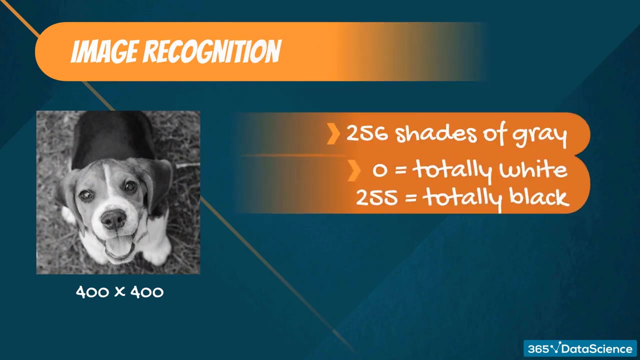 Given enough pixels and a big enough zoom-out, causes our brain to perceive this as an image rather than a collection of squares. Let's dig into that. Here's a simple grayscale photo. The grayscale contains 256 shades of gray, where 0 is totally white and 255 is totally black. 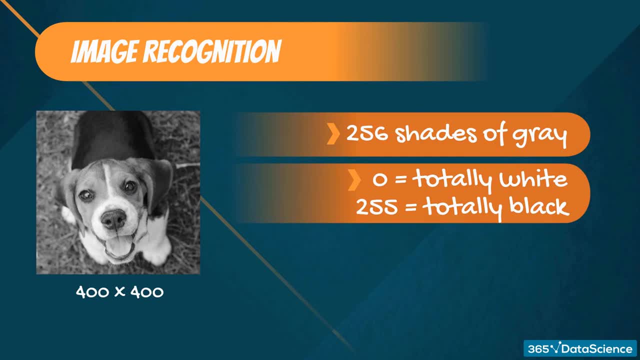 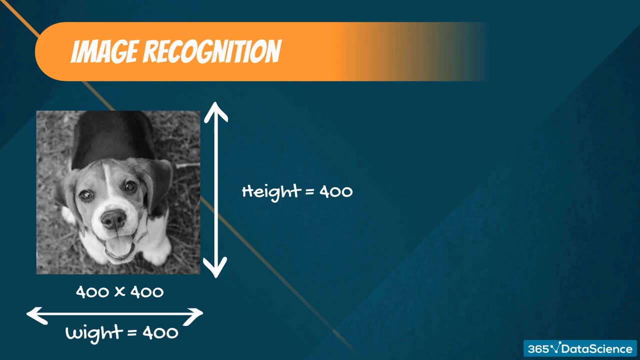 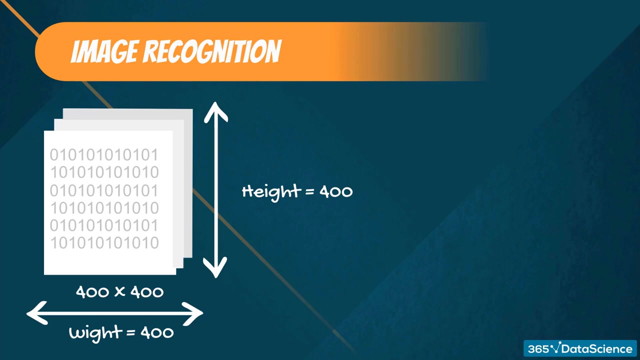 or vice versa. We can actually express this photo as a matrix. If the photo is 400 by 400, then that's a 400 by 400 matrix. Each element of that matrix is a number from 0 to 255.. It shows the intensity of the color gray in that. 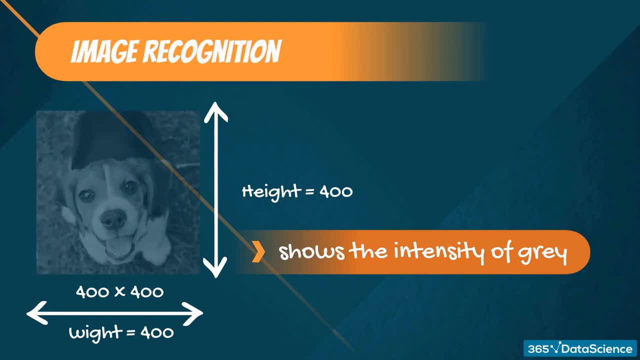 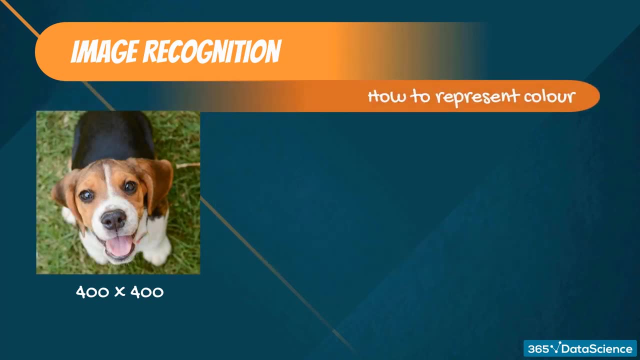 pixel. That's how the computer sees a photo, But grayscale is boring, isn't it? What about colored photos? Well, so far we had two dimensions: width and height, while the number inside corresponded to the intensity of color. What if we want more colors? Well, one solution: mankind. 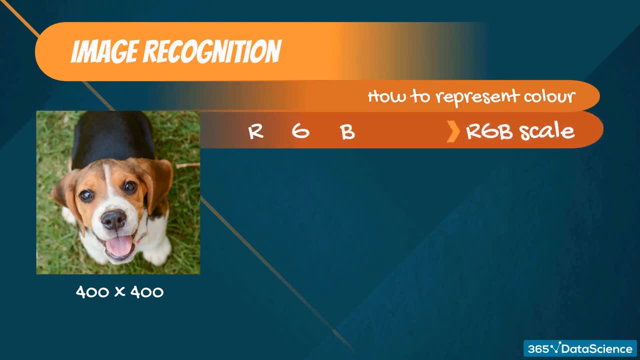 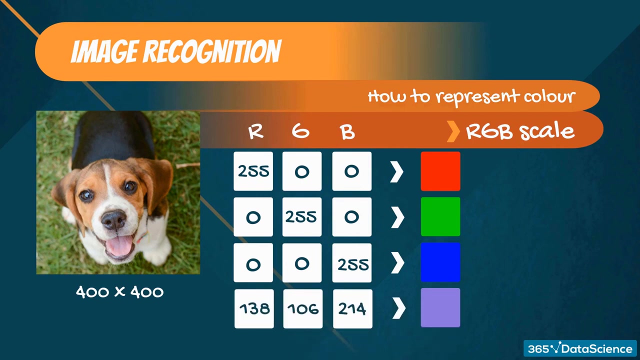 has come up with is the RGB scale, where RGB stands for red, green and blue. The idea is that any color perceivable by the human eye can be decomposed into some combination of red, green and blue, where the intensity of each color is from 0 to 255, a total of 256 shades. 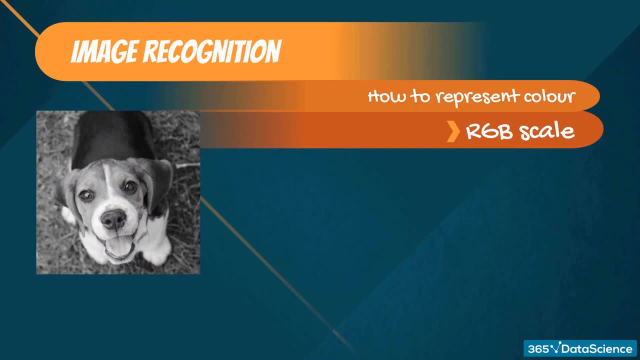 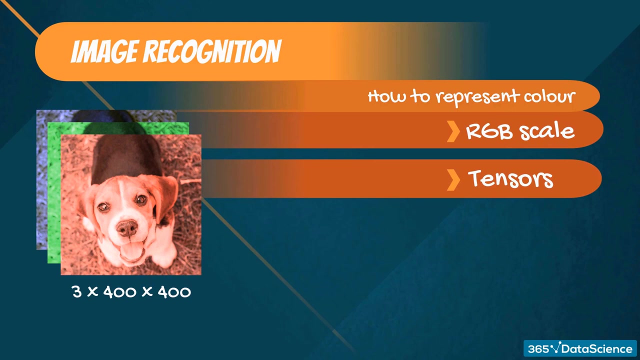 In order to represent a colored photo in some linear algebraic form, we must take the example from before and add another dimension- color. So instead of a 400 by 400 matrix, we get a 3 by 400 by 400 tensor. This tensor contains three 400 by 400 matrices. 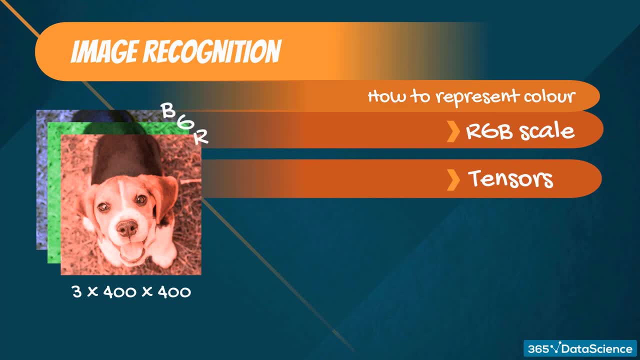 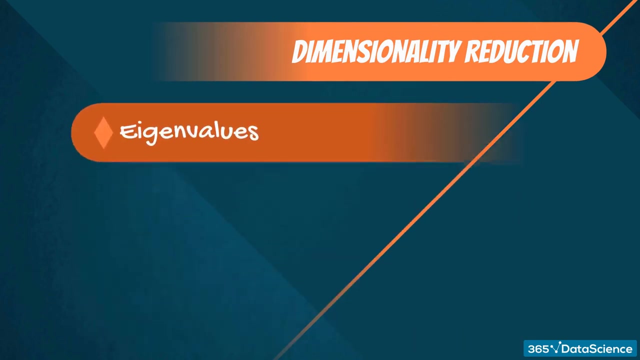 one for each color: red, green and blue- And that's how deep neural networks work with photos. Great, Finally, Dimensionality Reduction. Since we haven't seen Eigenvalues and Eigenvectors yet, there is not muchSíluciens. 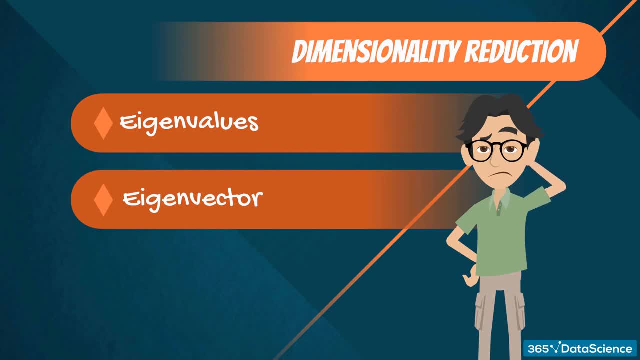 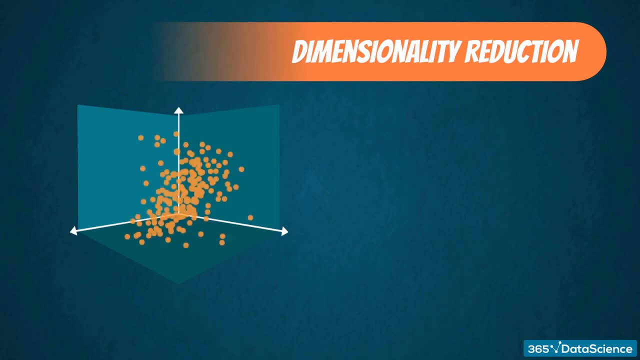 There is not much to say here, except for developing some intuition. Imagine we have a data set with three variables. Visually, our data may look like this: In order to represent each of those points, we have used three values, one for each variable: x, y and z. 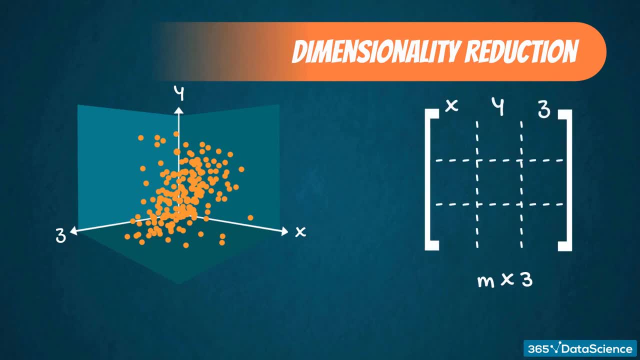 Therefore we are dealing with an m by 3 matrix, So the point i corresponds to a vector: x, i, y, i and z. i Note that those three variables, x, y and z, are the three axes of this plane. 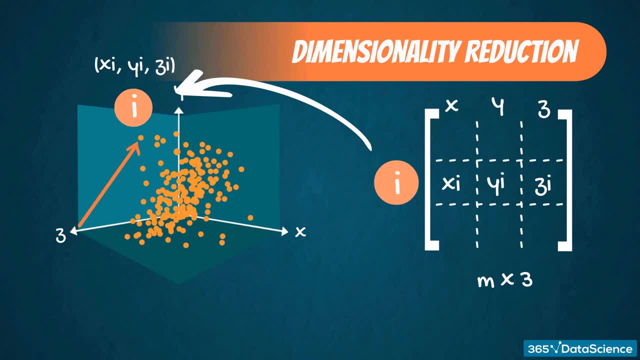 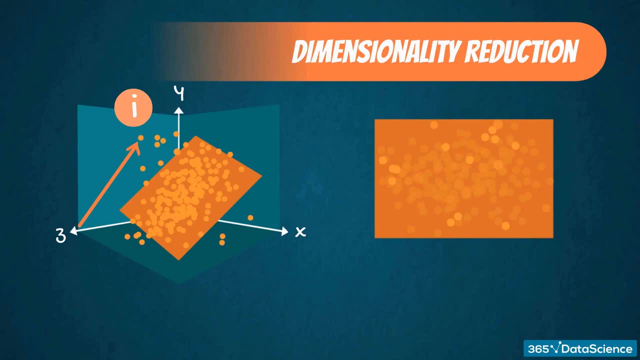 Here's where it becomes interesting. In some cases we can find a plane very close to the data, something like this: This plane is two-dimensional, so it is defined by two variables, Say u and v. Not all points lie on this plane, but we can approximately say that they do. 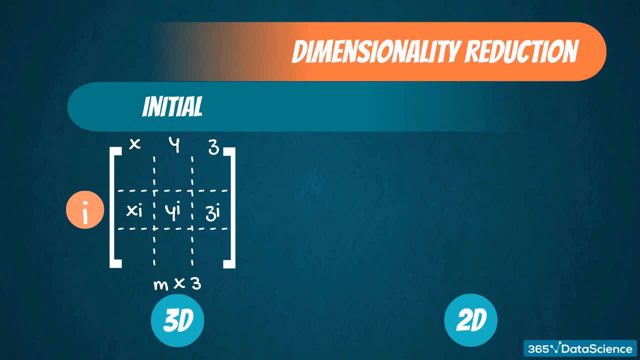 Linear algebra provides us with fast and efficient ways to transform our initial matrix from m by 3, where the three variables are x, y and z, into a new matrix, which is m by 2, where the two variables are u and v. 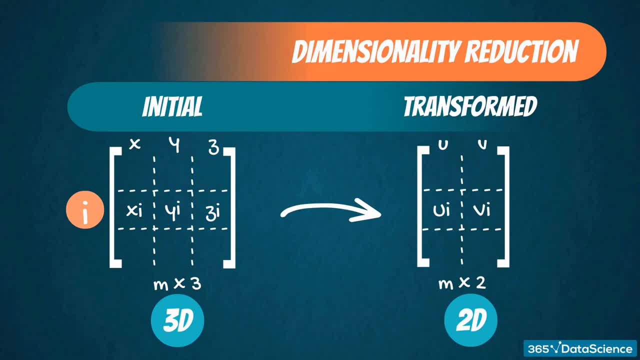 In this way, instead of having three variables, we reduce the problem to two variables. In fact, if you have 50 variables, you can reduce them to 40, or 20, or even 10.. How does that relate to the real world? 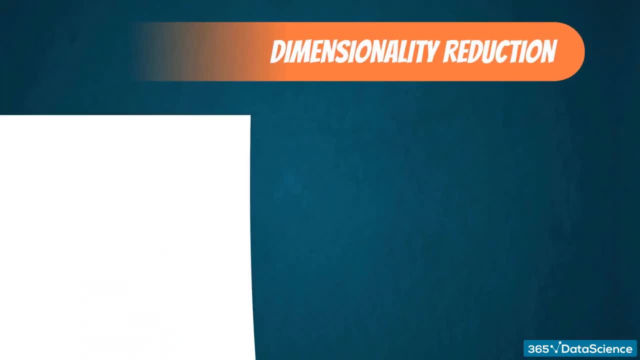 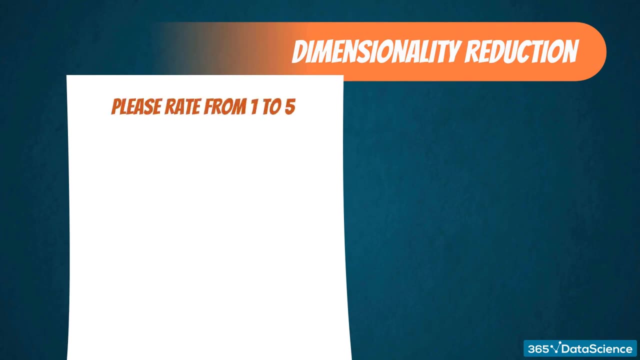 Why does it make sense to do that? Well, imagine a survey where there is a total of 50 questions. Three of them are the following. Please rate from 1 to 5.. 1. I feel comfortable around people. 2. I easily make friends. 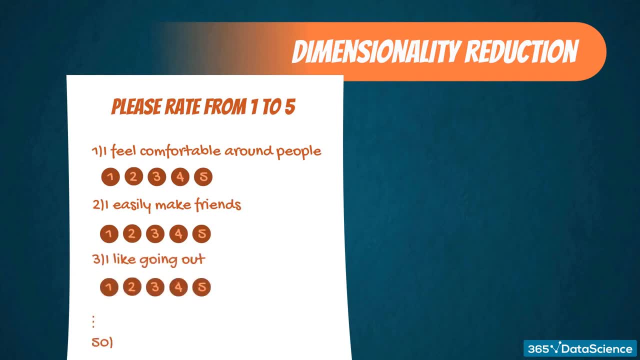 3. I have friends And 3. I like going out. Now, these questions may seem different, but in the general case they aren't. They all measure your level of extroversion, So it makes sense to combine them right. 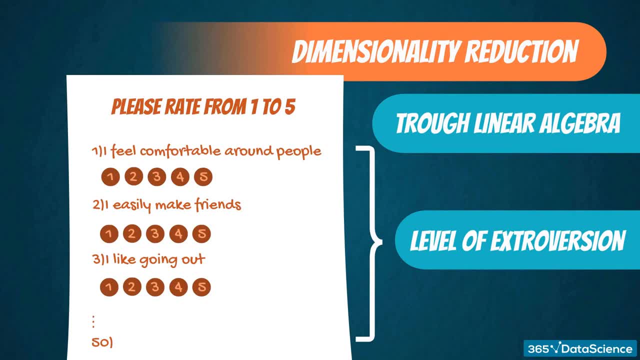 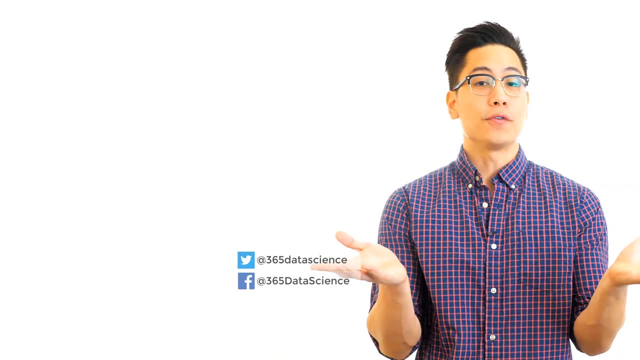 That's where dimensionality reduction techniques and linear algebra come in. Very, very often we have too many variables that are not so different, so we want to reduce the complexity of the problem by reducing the number of variables. Thanks for watching. If you found this video interesting and want to gain an edge in your career. 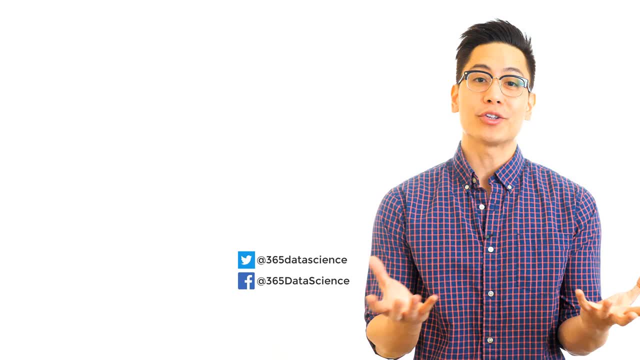 make sure to like, comment and subscribe, And don't forget to check out some of our other videos for another quick win in the data science skills department. 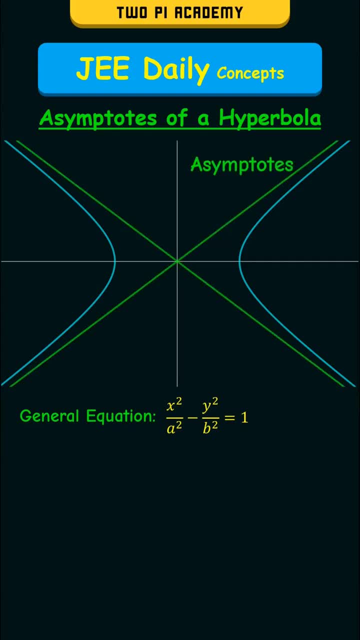 Asymptotes are one of the important concepts of hyperbola. But what does asymptotes mean? Asymptotes can be defined as the tangents of the hyperbola, as the point of contact tends to infinity, That is, they intersect: the hyperbola at infinity And the asymptotes of a hyperbola. 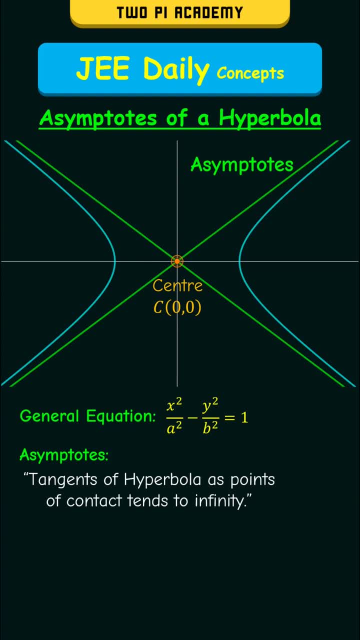 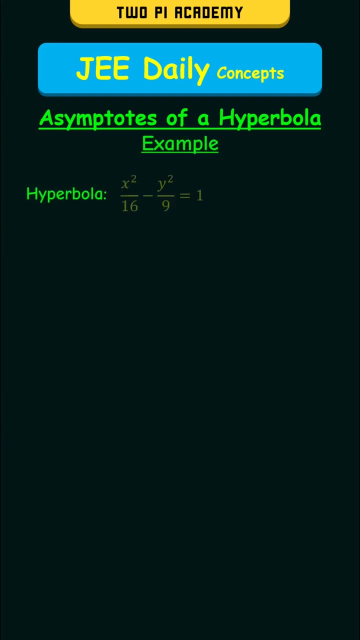 pass through the center of it, which is given by C in this case, And the equation of the asymptotes can be given by x square by a square minus y square by b square is equal to 0, or y is equal to plus or minus b, by a into x, For example. consider the hyperbola. 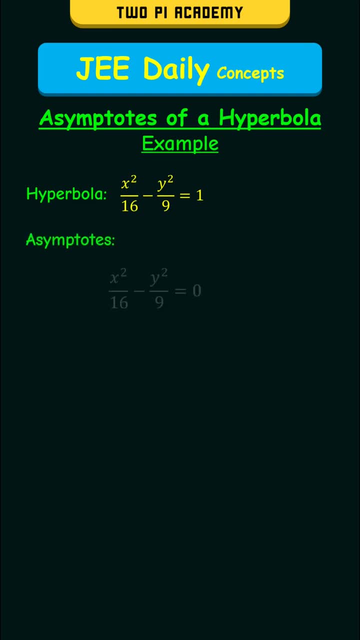 x square by 16 minus y square by 9, is equal to 1.. Then its asymptotes can be given by the equation: x square by 16 minus y square by 9 is equal to 0, or y is equal to plus or minus 16 by 9 into x. Please subscribe to the channel to not miss any future uploads.